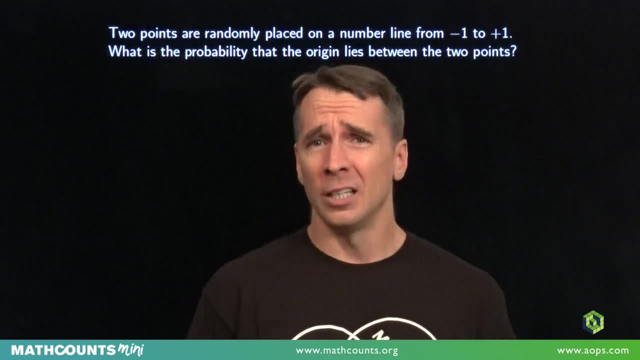 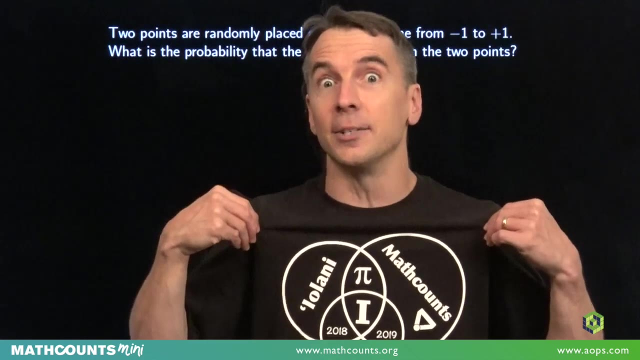 But here's the thing about probability problems: Sometimes they're a lot easier than they look. So step one, no fear. Step two: read the problem carefully, Dive right in. You might find out the water's pretty warm, just like it is in Hawaii. Now let's get to work. Two points: 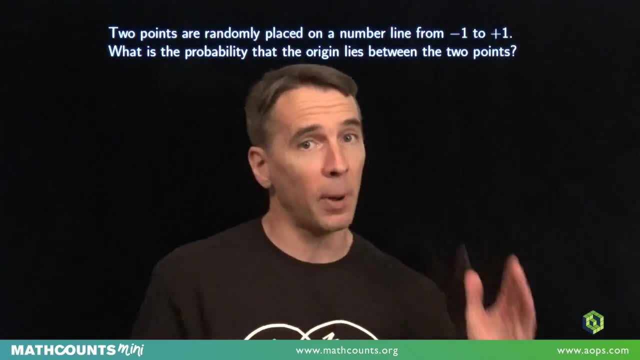 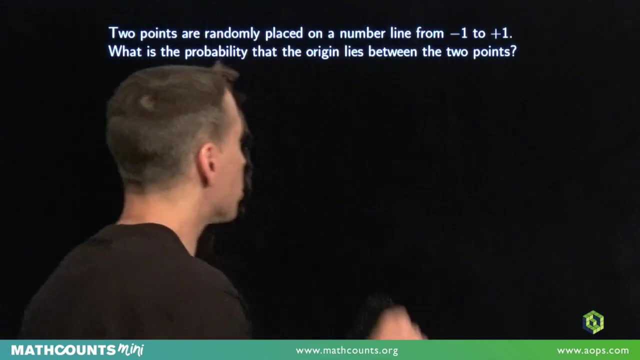 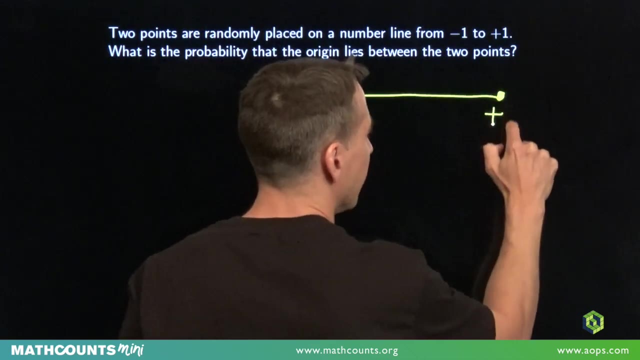 are randomly placed on a number line from negative one to positive one. We have to find the probability that the origin is between the two points that we choose. So let's draw that number line. The number line goes from negative one to positive one. 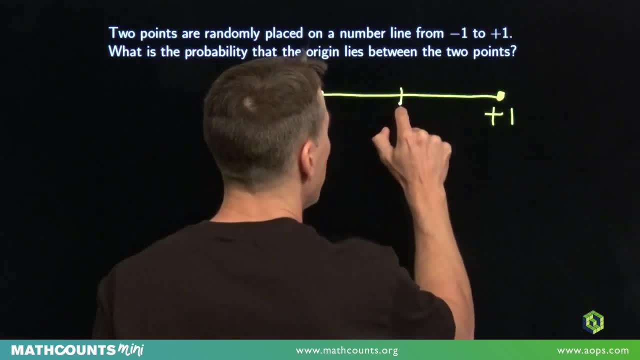 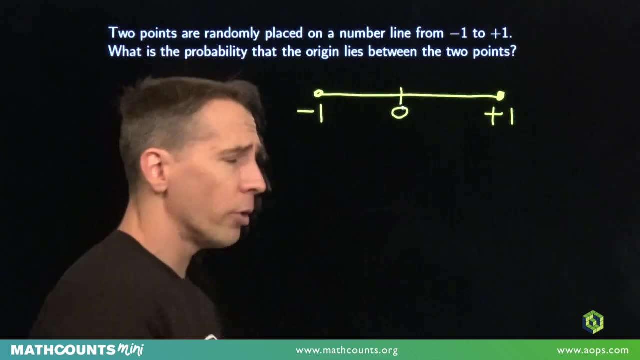 And we want the probability that the origin is between the two points that we're going to choose on this line. Origin that's zero, right there. So in order for the origin to be between our two points, one of them has to be to the left of zero, one of them has 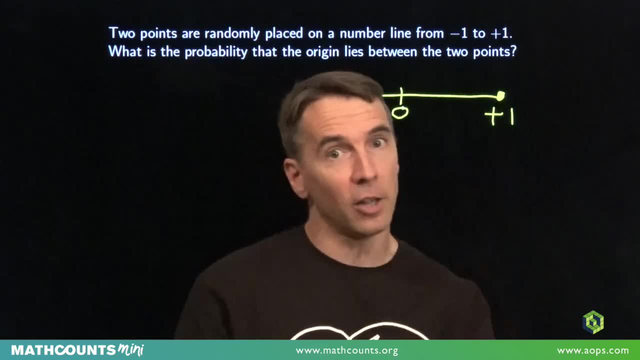 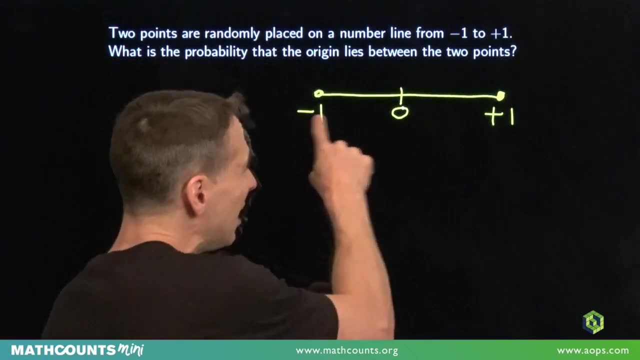 to be to the right of zero. So one has to be negative, the other has to be positive. Now we're not going to worry about choosing zero, because zero is just one point out of the infinitely many points between negative one and positive one. So the probability we'll 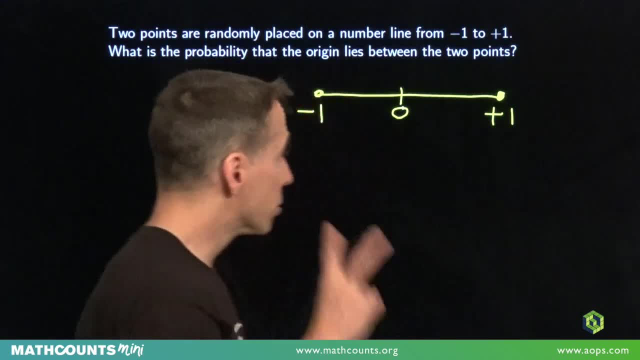 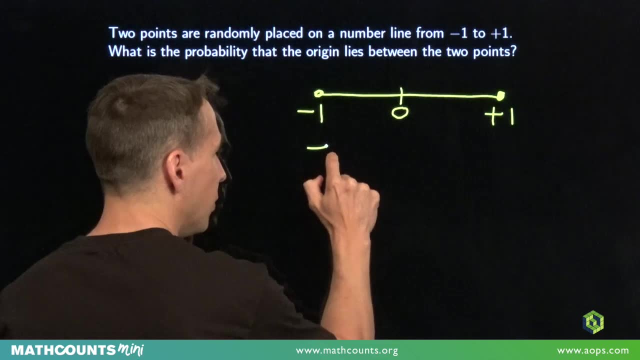 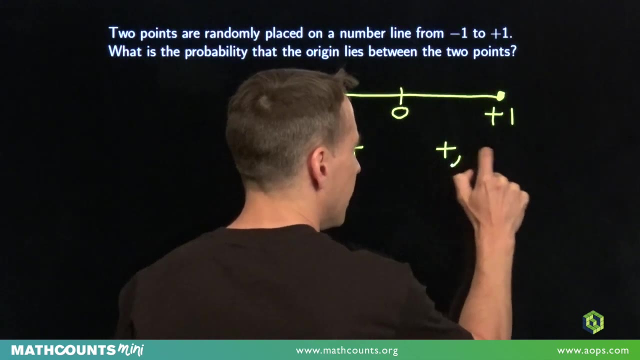 ever choose. zero is zero. Now, there are two ways we can end up with that zero. between the two points that we choose, We could choose a negative number first and then a positive number, or we could choose a positive number and then a negative number. So that's the. 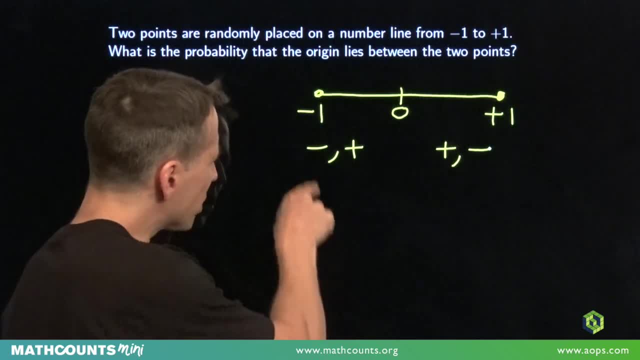 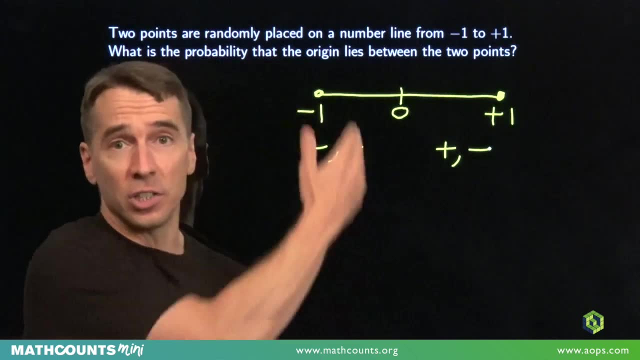 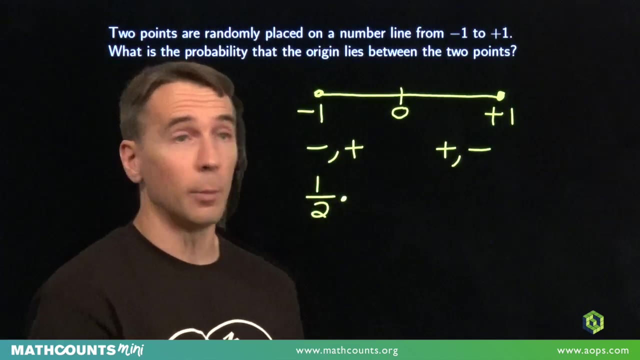 two ways. Let's take care of the first case. First case: we choose a negative number first. Probability of that happening is exactly half, because exactly half of this number line is negative. And then, for our second number, the probability- we'll choose a positive number. well, half. 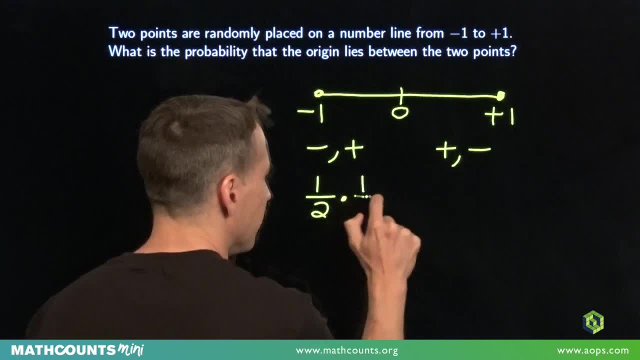 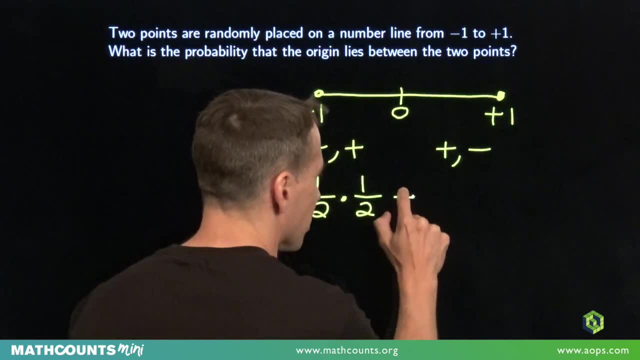 the number line is positive. So the probability we'll choose a positive number second is also a half. Now let's take a look at the other case. We choose the positive number first. We know that that happens with probability one half, because half the number line is. 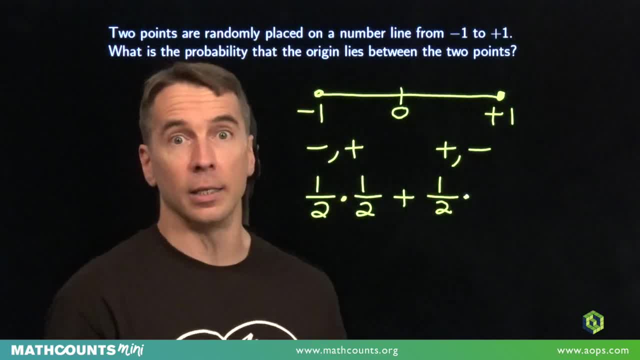 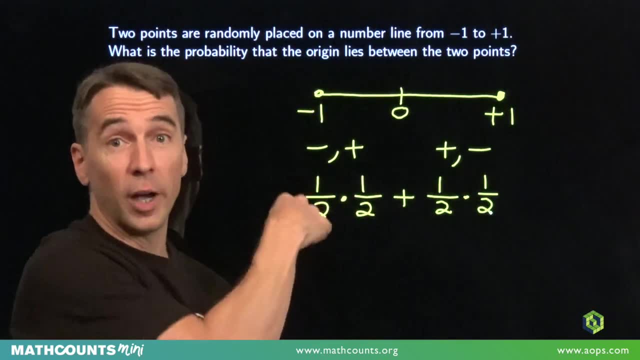 positive And then we choose the negative number. second, That happens with probability half, because half the number line is negative. So those are our two cases. We find the probability in each case, then add them up One half times one half, that's one quarter. 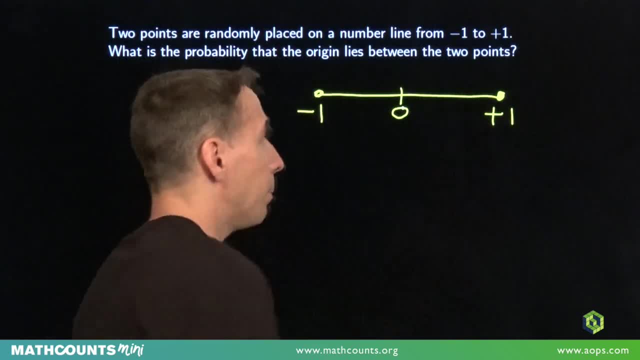 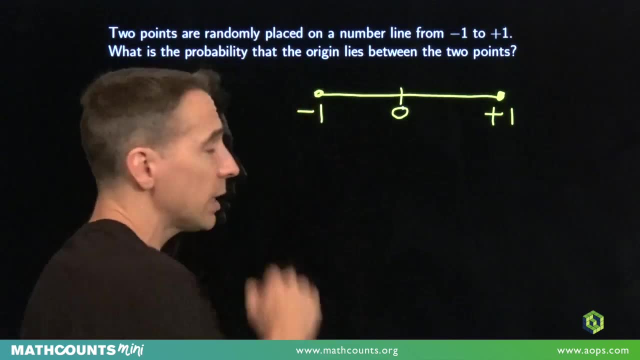 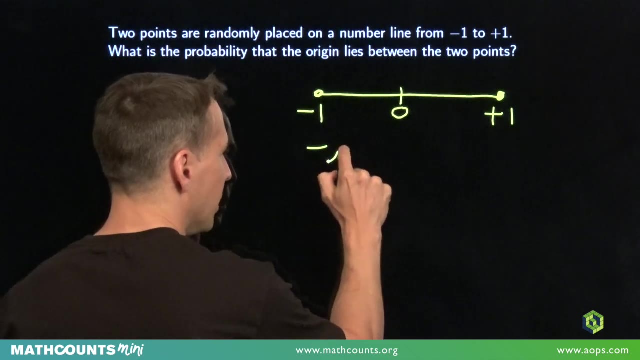 the infinitely many points between negative one and positive one. So the probability we'll ever choose zero is zero. Now there are two ways we can end up with that zero. between the two points that we choose, We could choose a negative number first and then a positive number, or we could choose 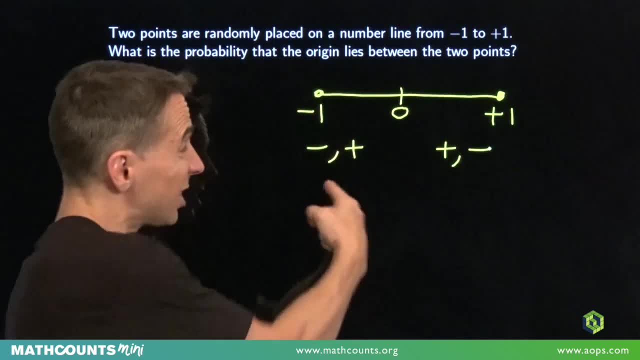 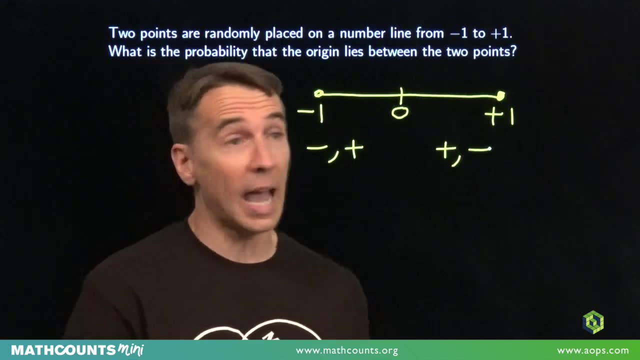 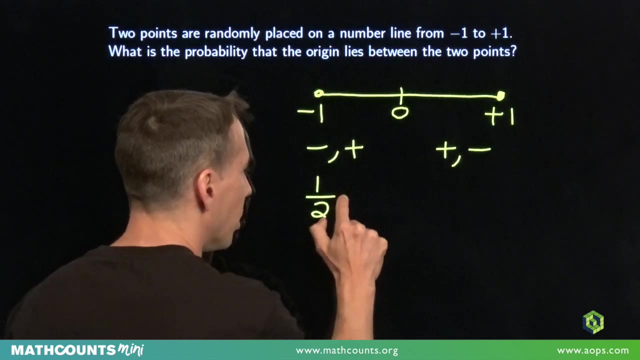 positive number and then a negative number. Subtitles by the Eagles. Let's take care of the first case. First case: we choose a negative number first. Probability of that happening is exactly half, because exactly half of this number line is negative. And then for our second number, the probability we'll choose a positive number. well, half. 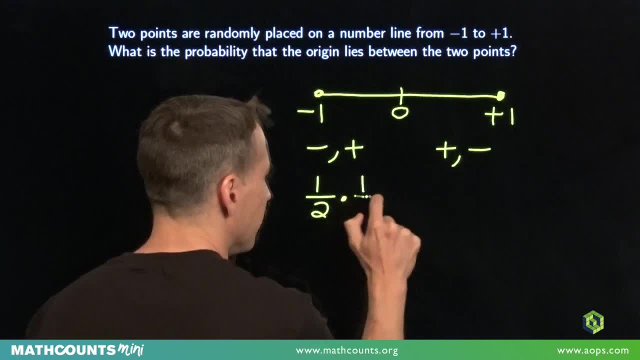 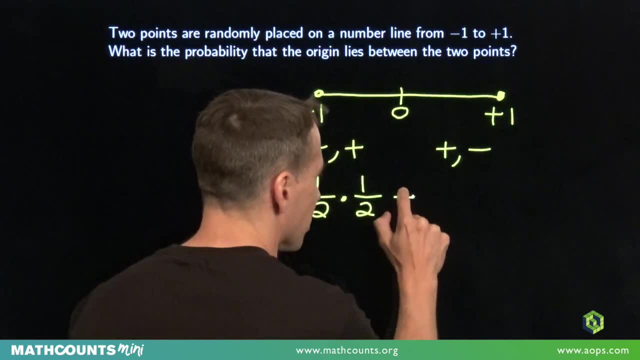 the number line is positive. So the probability we'll choose a positive number second is also a half. Now let's take a look at the other case. We choose the positive number first. We know that that happens with probability one half, because half the number line is. 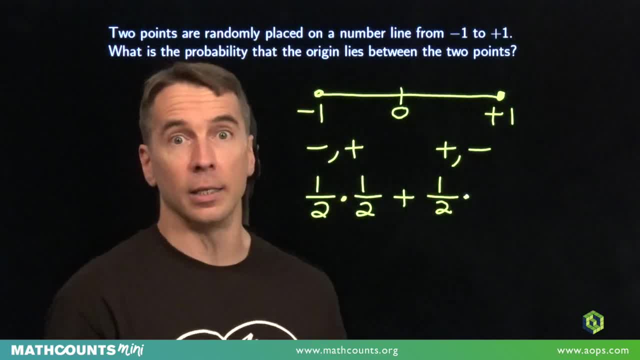 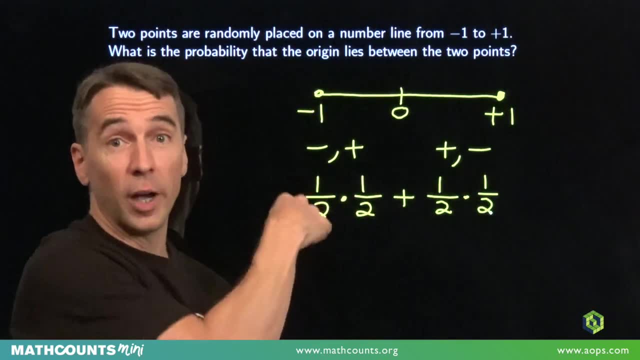 positive And then we choose the negative number. second, That happens with probability half, because half the number line is negative. So those are our two cases. We find the probability in each case, then add them up One half times one half, that's one quarter. 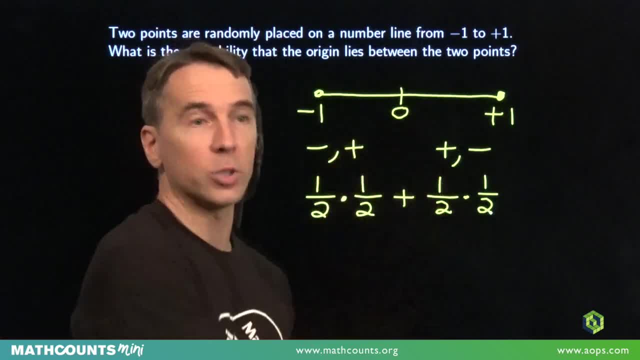 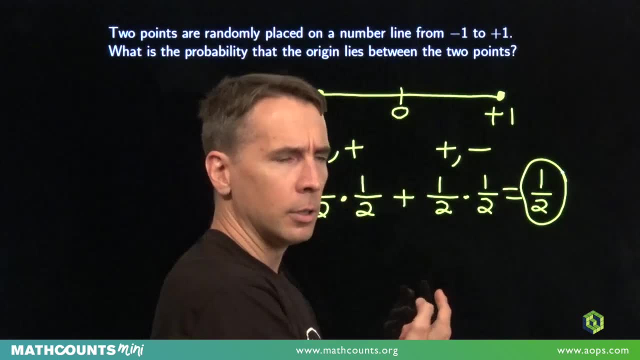 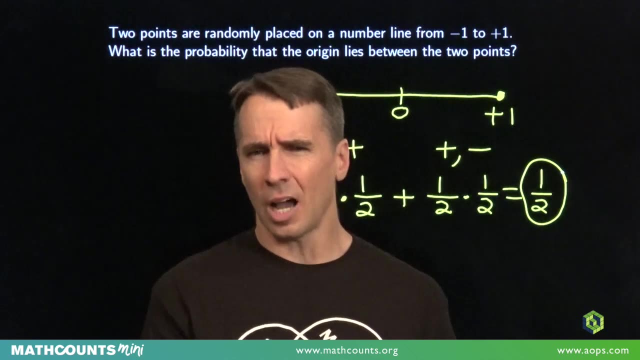 One half times one half, that's still one quarter. One quarter plus one quarter, our probability One half. Now I gotta tell you, whenever I see one half as the answer to a probability problem, I stop for a moment and I think maybe there's a faster way to solve this problem. 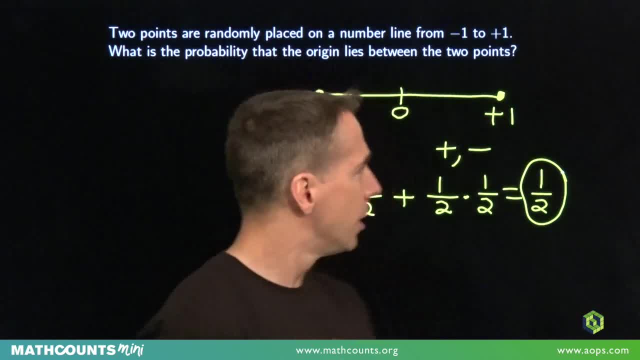 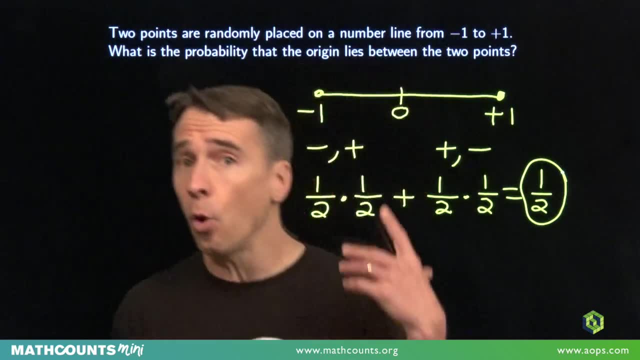 Maybe there's a nice slick way to see that the probability is a half. So we look back at our number line and we realize, no matter what we do in that first step, If we pick a negative or we pick a positive In our second step half. 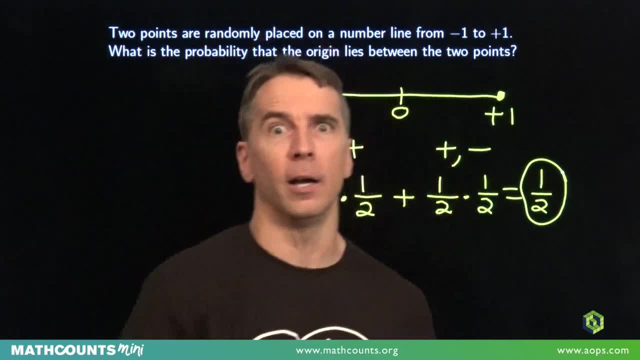 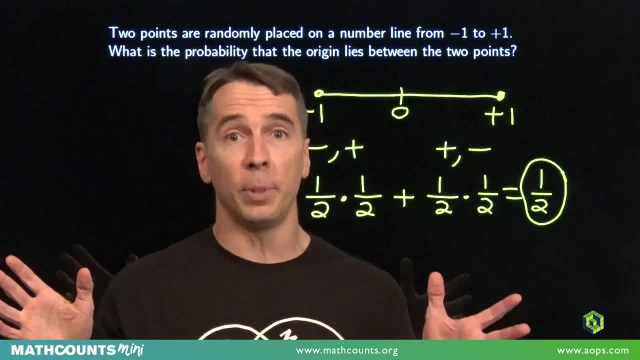 Yeah, half the time that second number's going to be on the other side of the origin, because half the number lines on the left, half the number lines on the right. So no matter what we pick first, half the time the next number's going to be on the other side. That's a much. 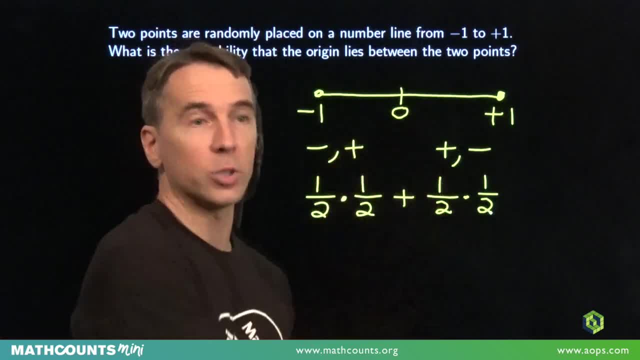 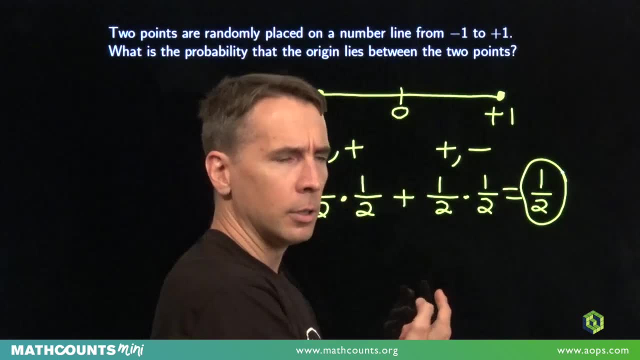 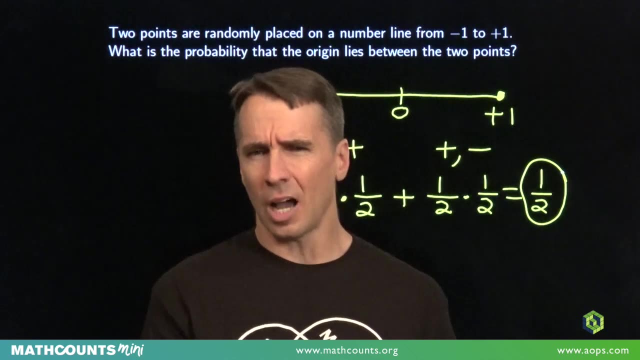 One half times one half, that's still one quarter. One quarter plus one quarter, our probability It's one half. Now I've got to tell you, whenever I see one half as the answer to a probability problem, I stop for a moment and I think maybe there's a faster way to solve this problem. 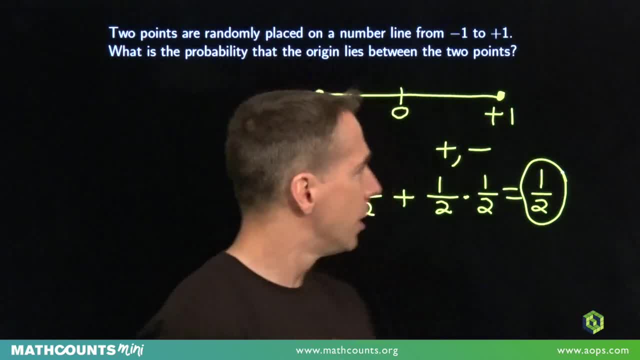 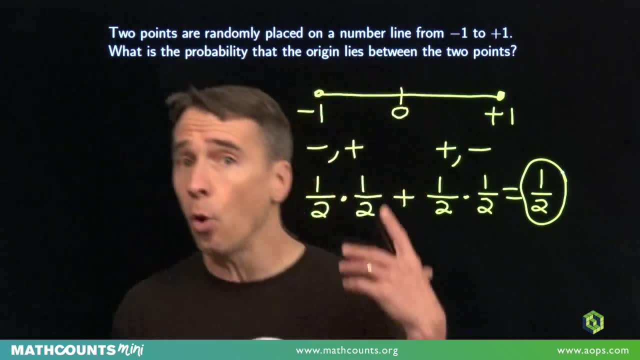 Maybe there's a nice slick way to see that the probability is a half. So we look back at our number line and we realize, no matter what we do in that first step, if we pick a negative or we pick a positive in our second step, half the number line is. 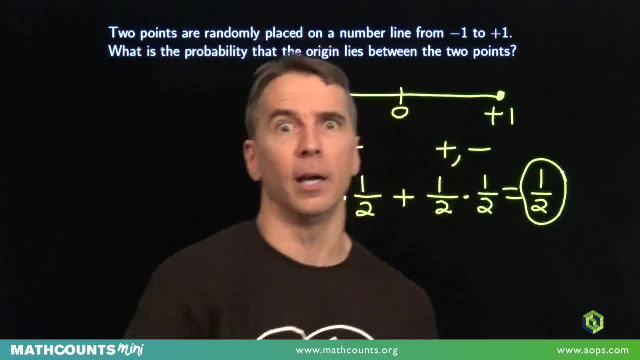 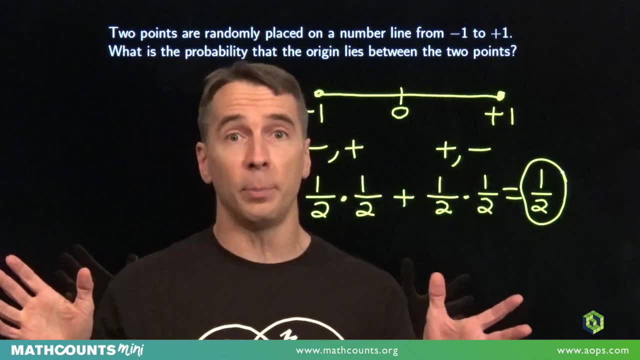 positive. Half the time that second number is going to be on the other side of the origin because half the number line is on the left, half the number line is on the right. So no matter what we pick first, half the time the next number is going to be on the 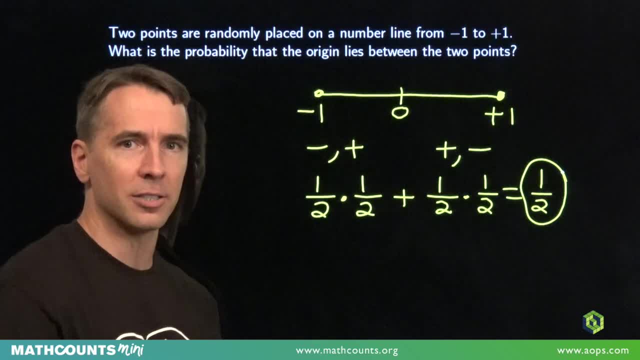 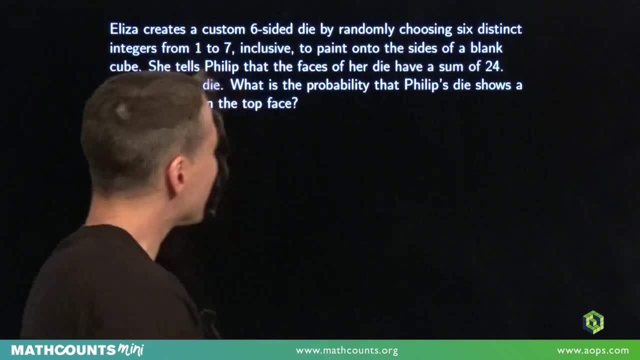 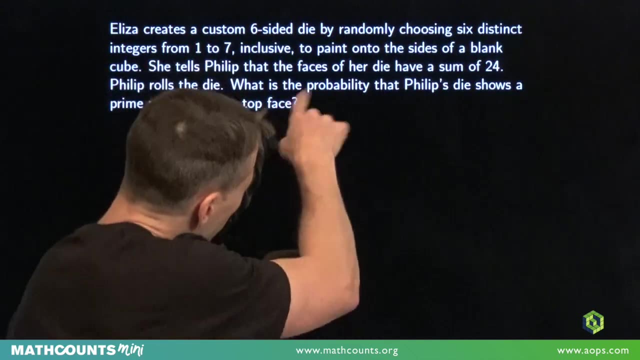 other side. That's a much nicer solution than all this, And we're ready for the second problem. All right, Eliza creates a custom six-sided die by randomly choosing six distinct integers, from one to seven, And then she's going to paint those on the side of a blank cube. 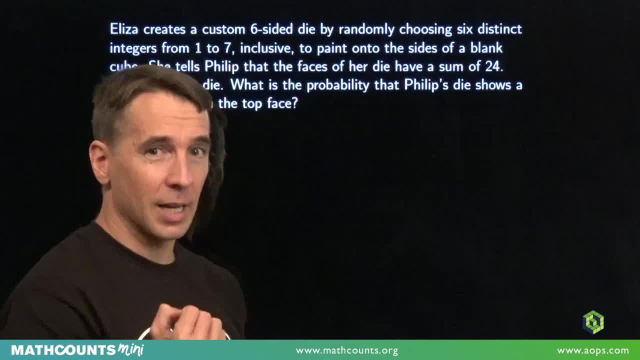 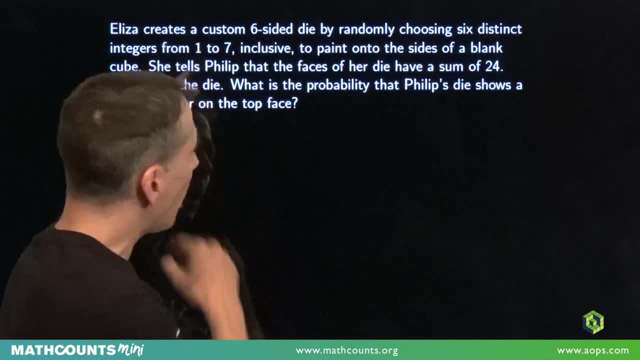 Then Phillip. well, Phillip's going to roll this die. She tells Phillip that the faces of her die have a sum of 24.. Phillip's going to roll that die and we want the probability that Phillip's roll shows a prime number up on top. 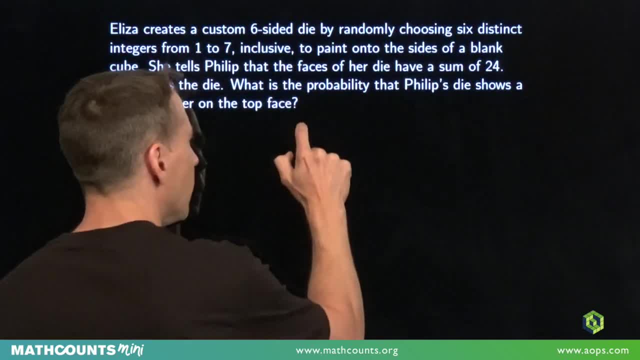 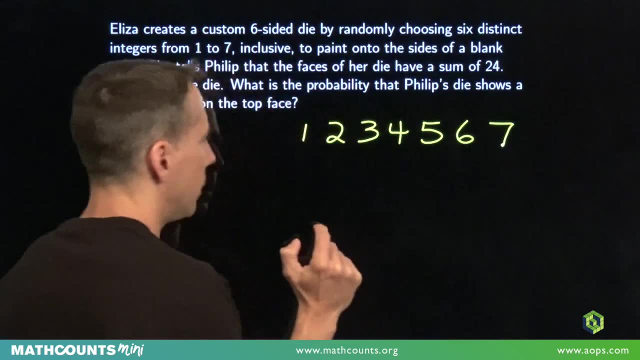 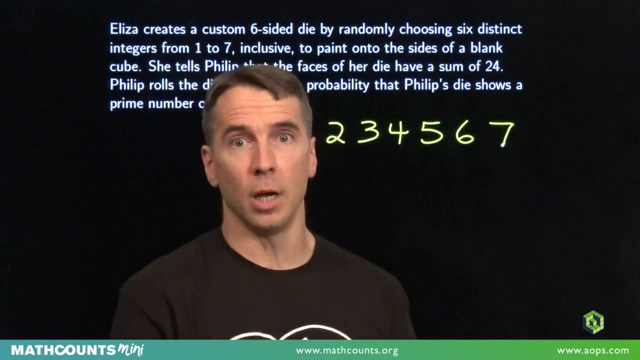 All right, where should we start? Well, we know she's going to make her die using numbers from one to seven. There are seven numbers there, only six sides of the cube, so we have to get rid of one of these numbers. 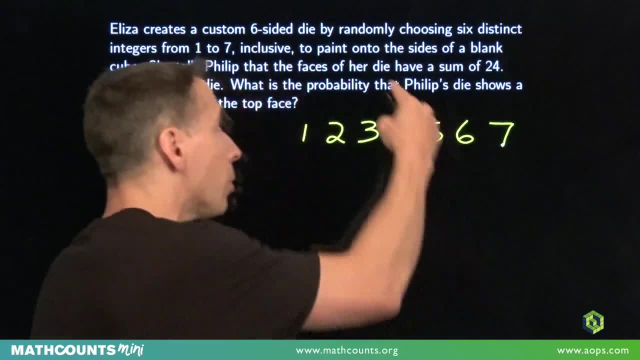 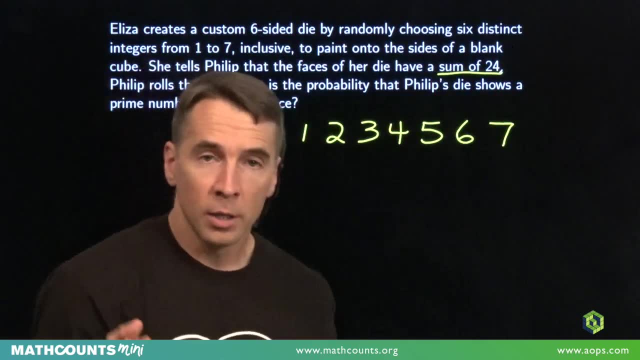 Now, if we don't see right away which number she's going to get rid of, we look back at the problem for information we haven't used yet We haven't used this sum of 24.. The six numbers that are on this die. they add up to 24, so we have to figure out which. 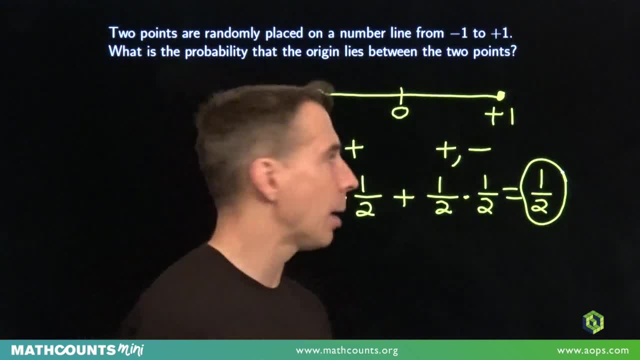 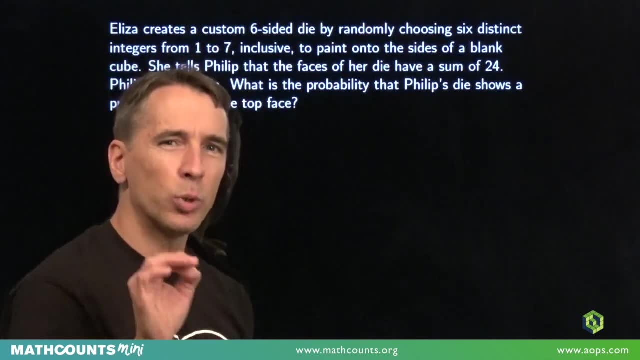 nicer solution than all this, And we're ready for the second problem. All right, Eliza creates a custom six-sided die by randomly choosing six distinct integers, from one to seven, And then she's going to paint those on the side of a blank cube. Then 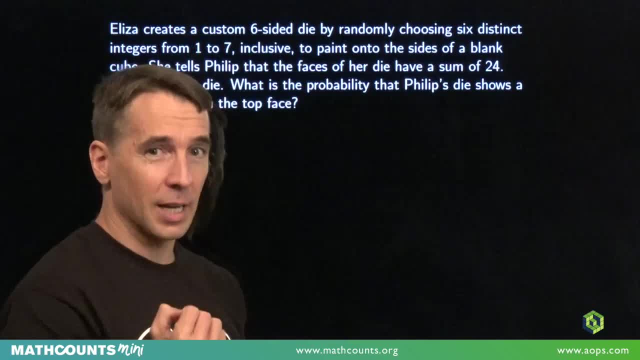 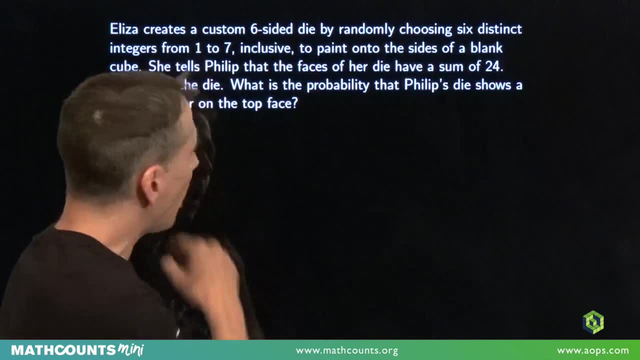 Philip. well, Philip's going to roll this die. She tells Philip that the faces of her die have a sum of twenty-four. Philip's going to roll that die and we want the probability that Philip's roll shows a prime number up on top. 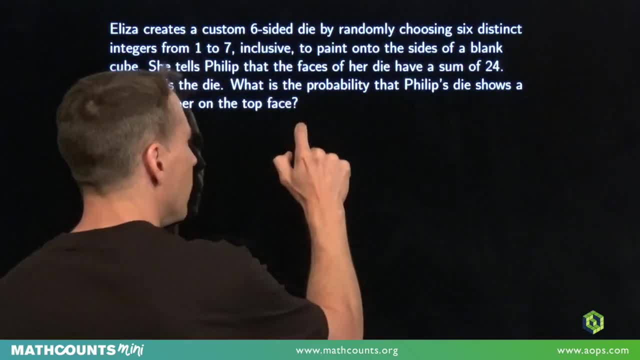 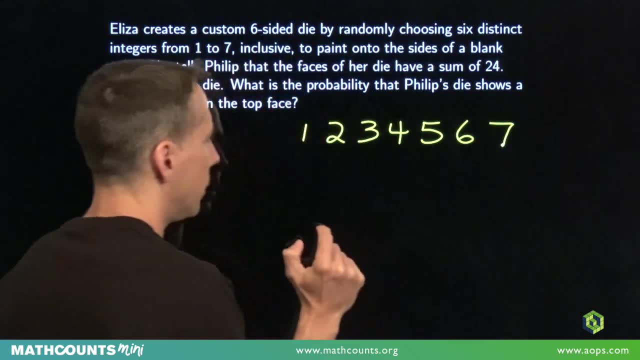 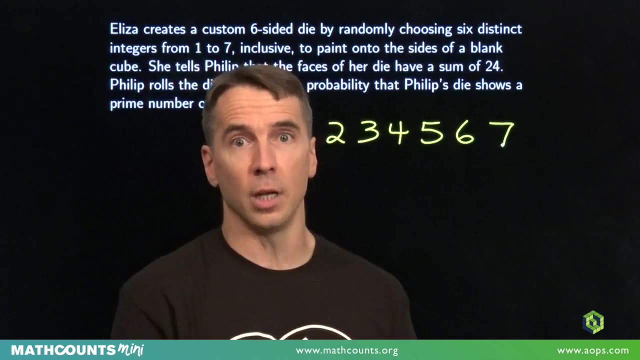 All right, where should we start? Well, we know she's going to make her die using numbers from one to seven. There are seven numbers there, only six sides of the cube, so we have to get rid of one of these numbers. Now, if we don't see right away which number she's going to get rid of. 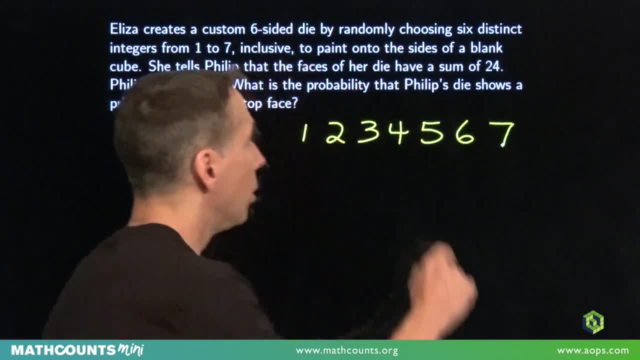 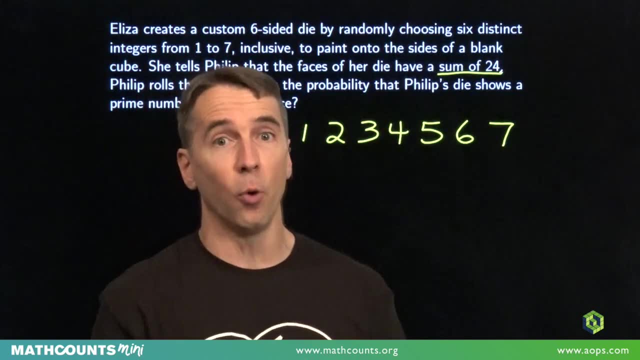 we look back at the problem for information we haven't used yet. We haven't used this sum of twenty-four, The six numbers that are on this die. they add up to twenty-four. so we have to figure out which six of these add up to twenty-four. 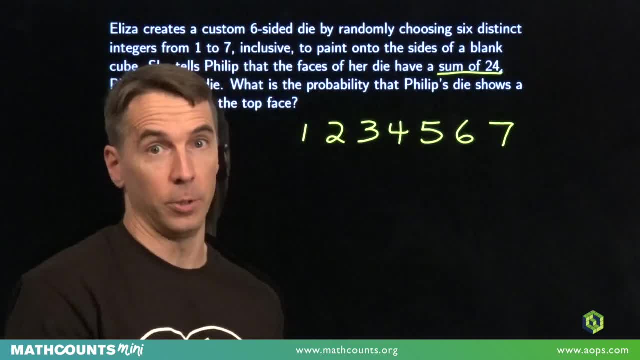 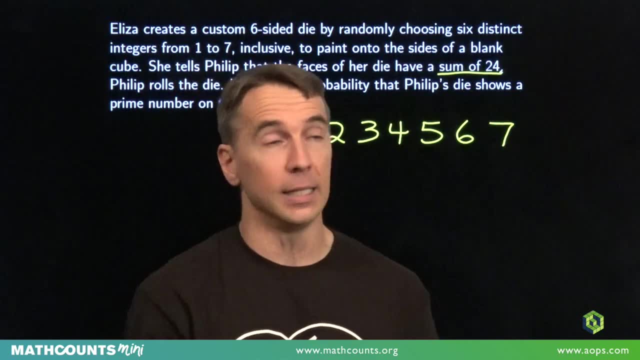 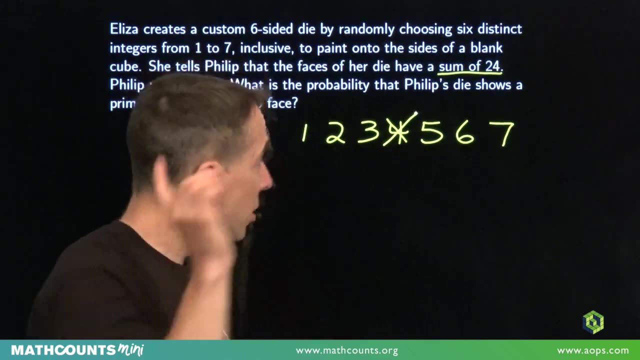 First we'll figure out what all seven of them add up to. These four here add up to ten. These three out there add up to eighteen. Put that together, you got twenty-eight. We only need twenty-four. so let's get rid of the four That will get us down to twenty-four. 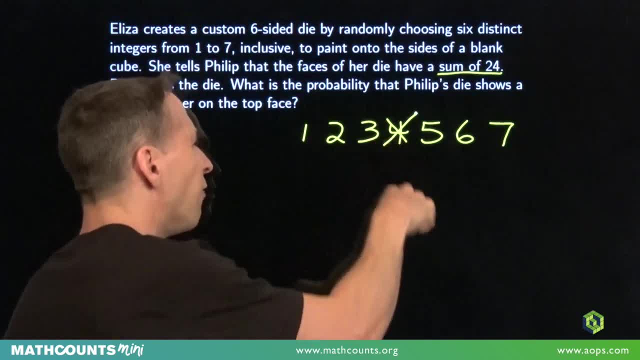 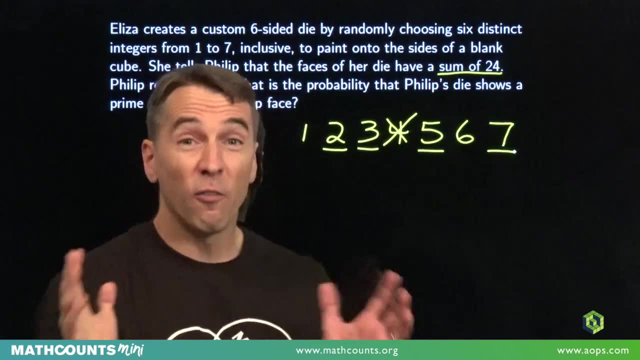 So the die that Philip is going to roll has a one, a two, a three, a five, a six, a seven. The prime numbers are two, three, five and seven, Four prime numbers out of here. They're numbers out of 6 total. So when he rolls that die, the probability he's going to get a prime 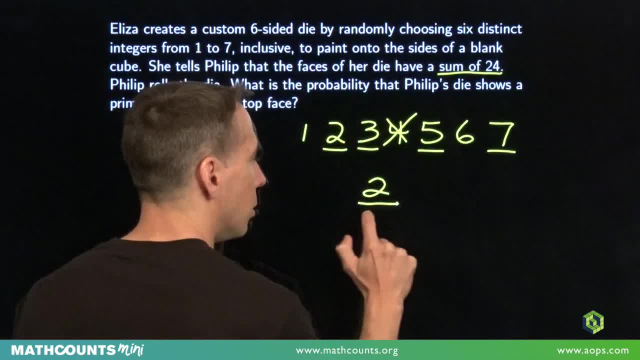 is 4 sixths, which you know is 2 thirds. Don't be afraid of probability problems.